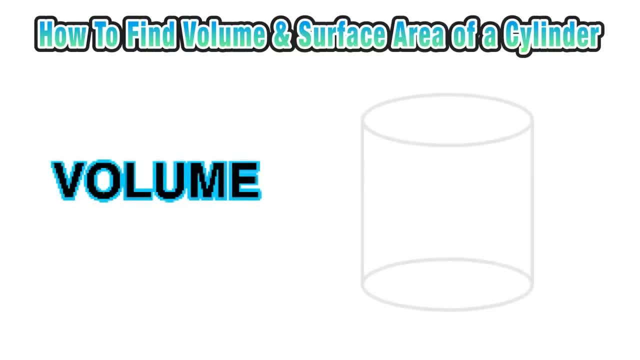 Now we know that volume represents the amount of space inside of a closed figure. So we can think of the volume of a cylinder as how much it can hold inside. maybe if we were to fill up a bucket with green paint, And we know that surface area represents the amount of space it would take to cover up, 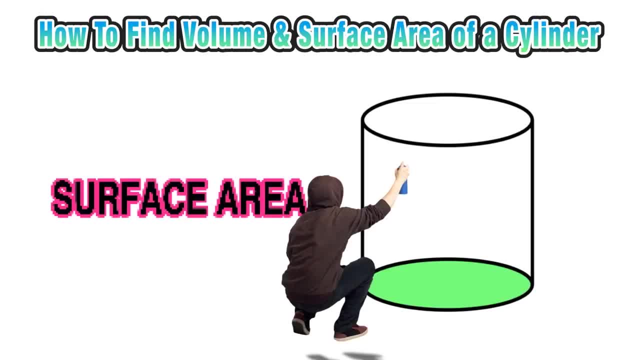 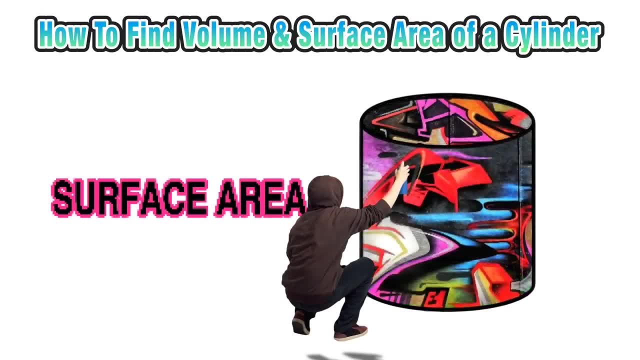 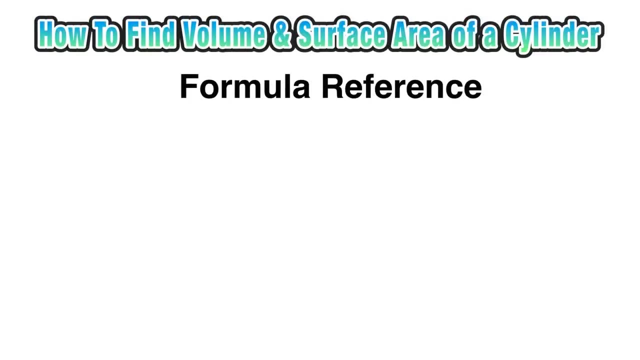 the outside of a figure, like if we were going to wrap it with wrapping paper or maybe spray paint it with some kind of a design. So now we're ready to go ahead and familiarize ourselves with the formulas for finding both volume and surface area of a cylinder. 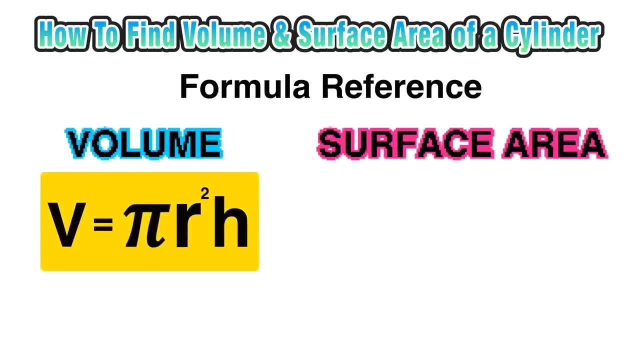 The volume of a cylinder can be found by multiplying pi times the radius squared times. the height And surface area can be found by multiplying the prime times, the square times. the height And surface area can be found by multiplying the prime times, the square times, the height. 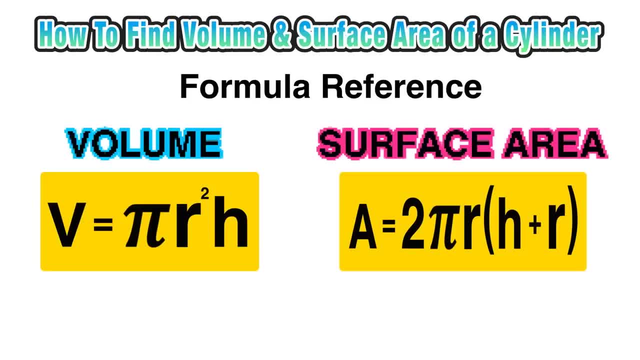 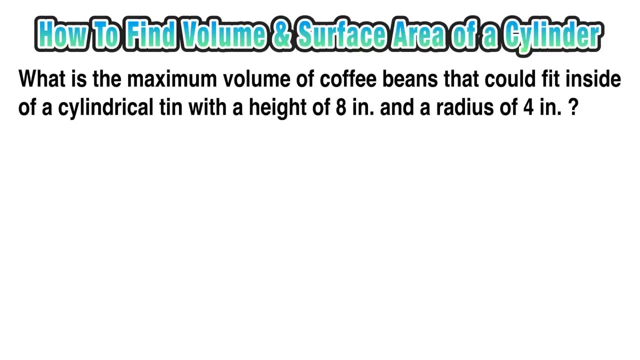 And remember that volume is measured in cubic units and surface area will be measured in square units. Ok, so now we're ready to take a look at this example, which is: what is the maximum volume of coffee beans that could fit inside of a cylindrical tin with a height of 8 inches? 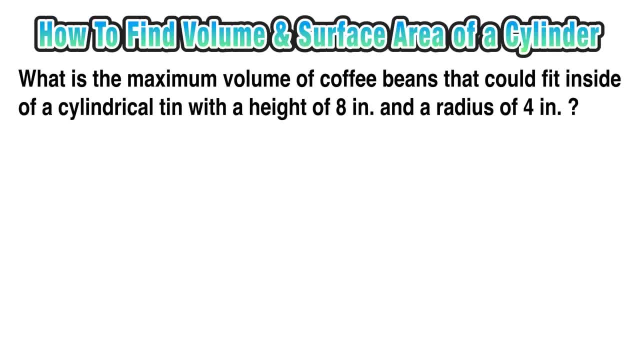 and a radius of 4 inches. Highlight. the key information in this case is that we want to find the volume of the inside of a cylinder with a height of 8 and a radius of 4.. So to visualize this, we're thinking about how many coffee beans can fit inside of a 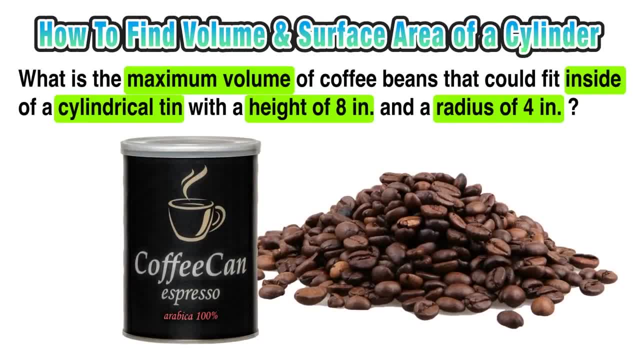 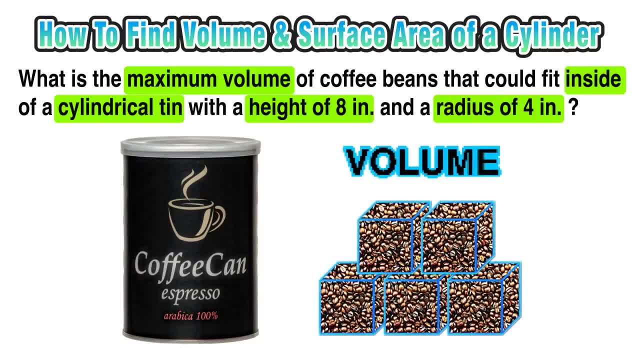 cylinder shaped can, And since we measure volume in cubic units, we're actually thinking of this, our answer, in terms of how many 1 inch cubes of coffee could fit inside of this can. So at this point we can revert back to that simple diagram of a cylinder. 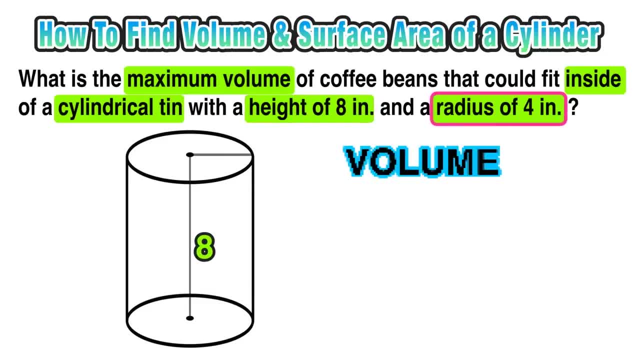 And we know that the height is 8, so we can label the height with the value of 8.. And the radius is 4 inches, so we can label the radius with a 4.. And now we can use our volume formula. v equals pi r squared h. 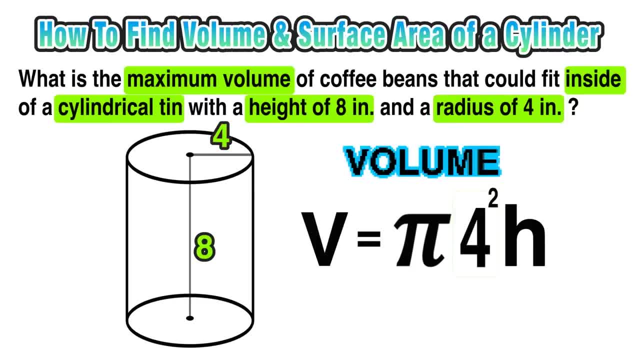 We can replace r squared with 4 squared, since the radius is 4.. And we know that 4 squared is just 16.. Then we can replace h, the value of the height, with 8, since the height was 8 inches. 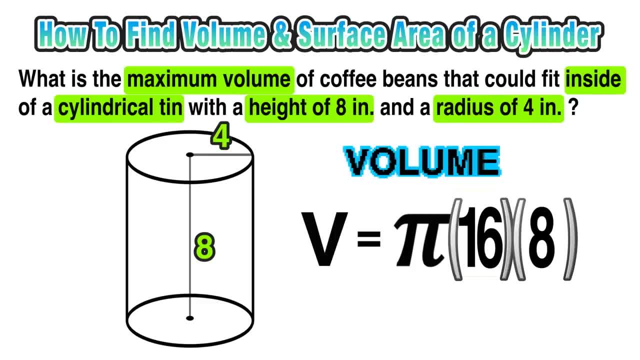 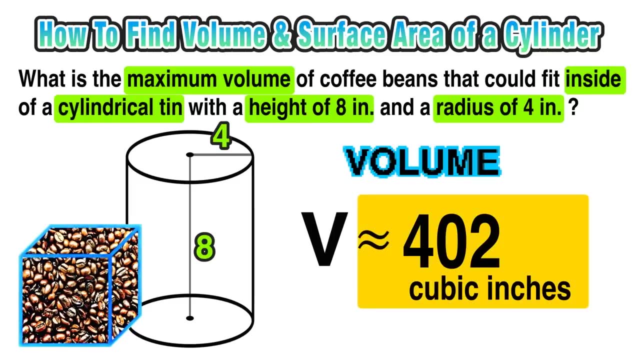 And now all we have to do is multiply To get our final answer. pi times 16 times 8 is approximately 402 cubic inches, and remember that means that this can could hold approximately 402 of these little 1 inch cubes of coffee. 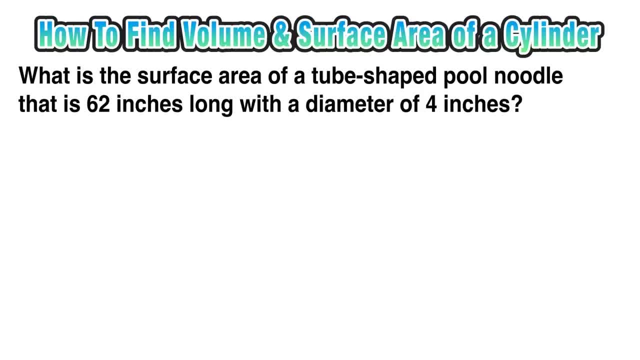 And now we have time for one more example Here. we want to know what is the surface area of a tube shaped pool noodle that is 62 inches long With a diameter of 4 inches. Now, the key information here is that we are looking for the surface area of a cylinder. 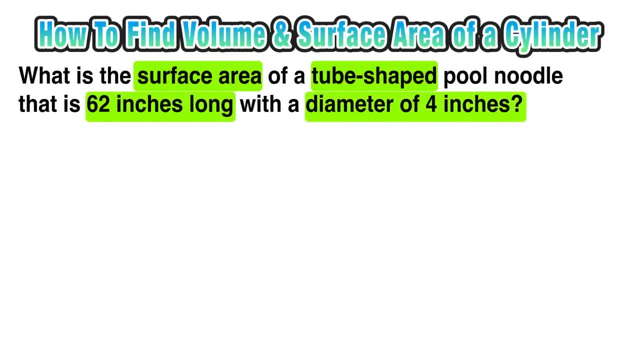 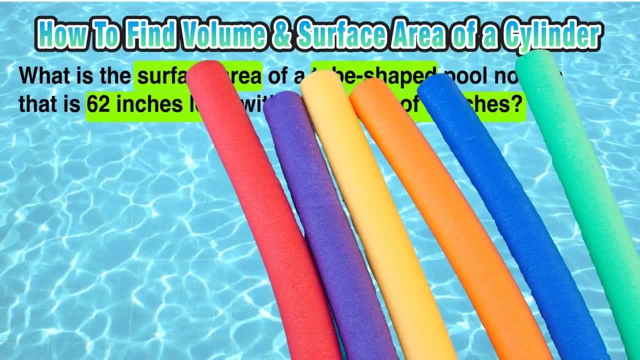 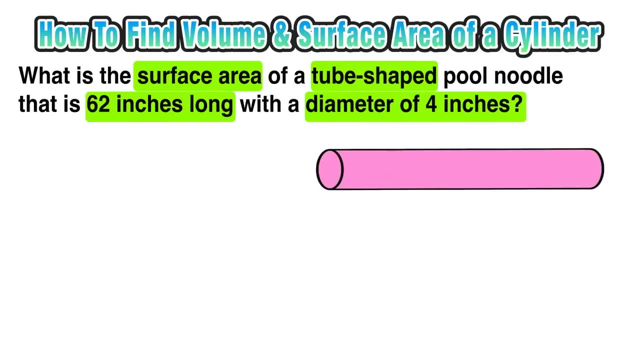 that is 62 inches long with a diameter of 4.. First, let's make sure that everyone knows what a pool noodle looks like. I know they are kind of dumb, just don't worry about it. So we have this pool noodle, which is really just a long skinny cylinder, and we want to 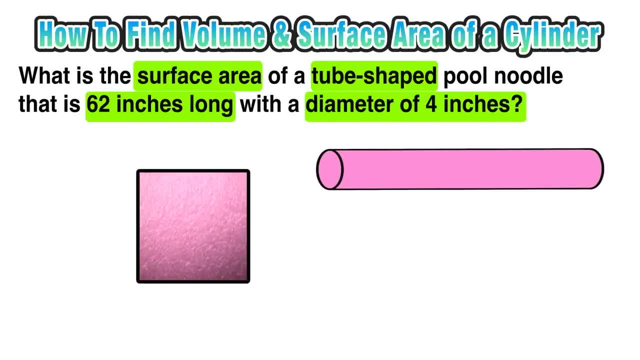 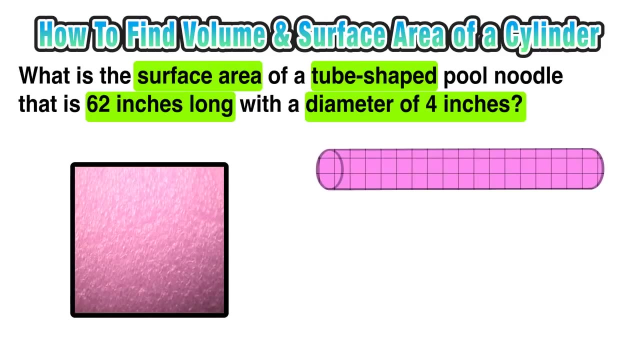 find surface area, Which really just means How many of 1 inch by 1 inch squares will it take to cover the entire outside of this pool noodle? Hence the reason why we measure surface area in square units. So now that we got the concept down, let's move on to the procedure. 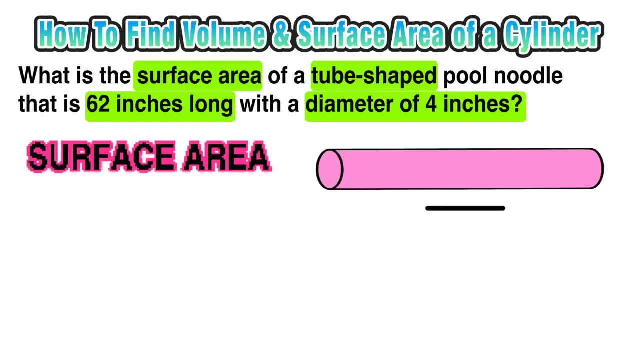 Now to find surface area. we can start off by labeling the diagram. We know that the length of the pool noodle is 62 inches and we know that the diameter of the circle Of the base is 4 inches, And we also know that the diameter is twice the length of the radius. 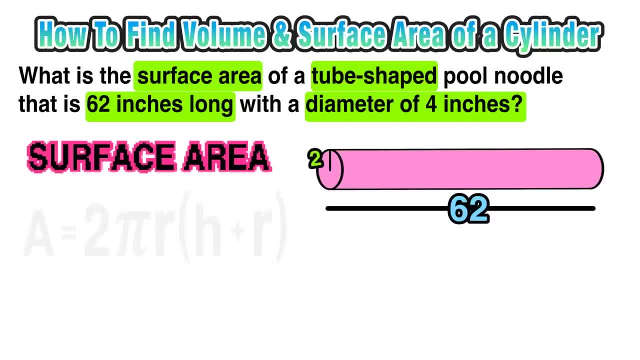 So half of 4 equals 2,, which is the radius that we need in order to use the formula Which we can now apply. Now we are going to go ahead and replace the radius, the r values, with 2,, since the radius 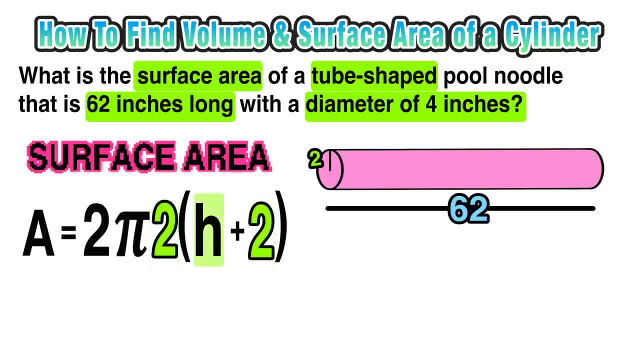 was 2.. And the length is the same thing as the height, So we can replace h with 62 in the formula. And now we can go ahead and evaluate this. And the surface area of this pool noodle is approximately 804 inches squared.